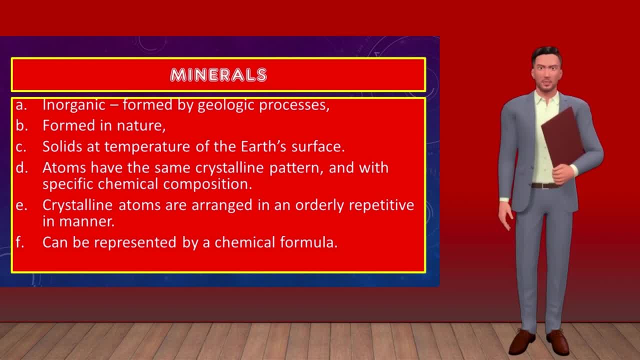 The minerals that make up rocks are called rock forming minerals. Only a few minerals are rock forming. Minerals can be described as: a- Inorganic, which formed by natural geologic processes. b- Formed in nature. c- Solids- The crystalline substance, are solid at temperature of Earth's surface. 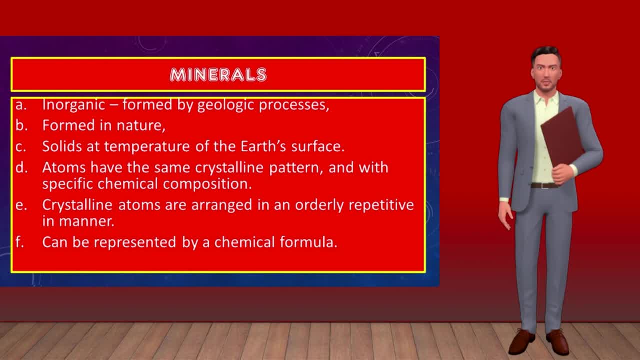 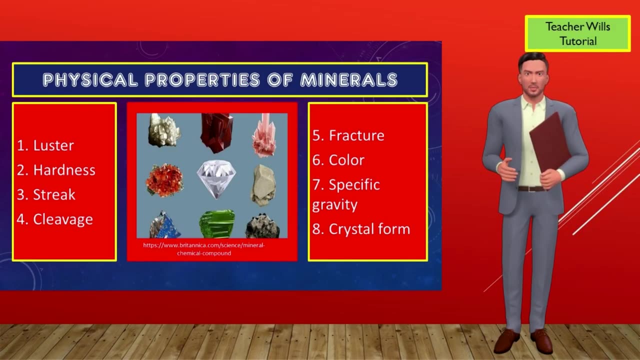 d Atoms have the same crystalline pattern and with specific chemical composition. e Crystalline atoms are arranged in an orderly, repetitive manner and f Can be represented by a chemical formula. The physical properties of minerals: Scientists identify more common minerals by their colors or appearances. others include their taste, smell, feel and sound. 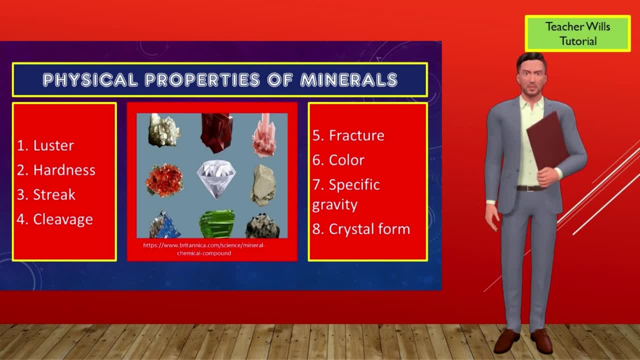 The physical properties of minerals that can be tested are: 1. Luster, 2. Hardness, 3. Streak, 4. Cleavage, 5. Fracture, 6. Color, 7. Specific gravity and 8. Crystal form or crystal habit. 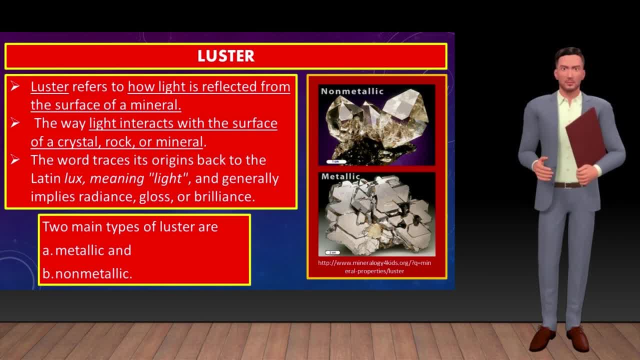 One of the physical properties of minerals is the lustre. Lustre refers to how light is reflected from the surface of a mineral. It is the way light interacts with the surface of a crystal, rock or mineral. The word traces its origins back to the Latin word. 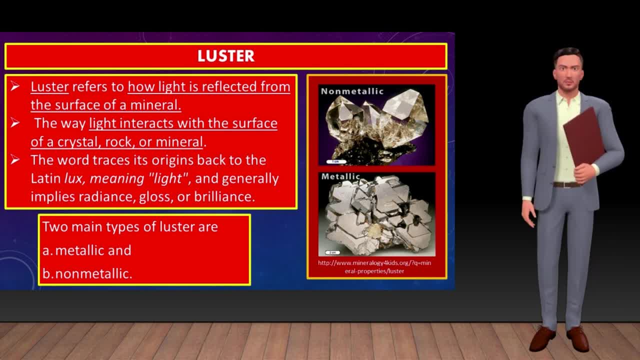 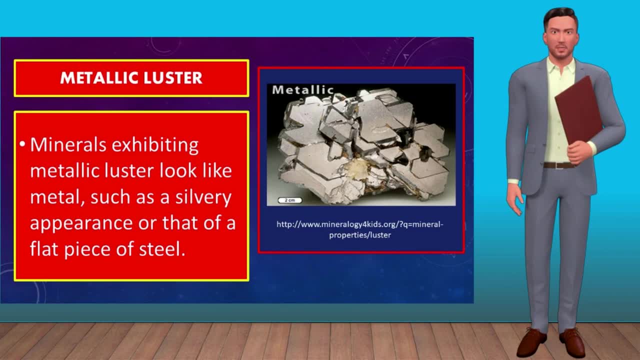 lux, meaning light, and generally implies radiance, gloss or brilliance. The two main types of lustre are metallic and nonmetallic. The metallic lustre: Minerals exhibiting metallic lustre look like metal, such as a silvery appearance or that of a flat piece of steel. 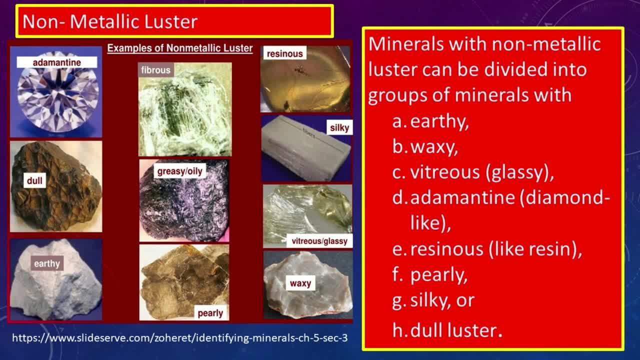 The nonmetallic lustre. Minerals with nonmetallic lustre can be divided into groups of minerals with a- Earthy, b Waxy, c, Vitreous or glassy. We also have d, Adamantine or diamond-like. 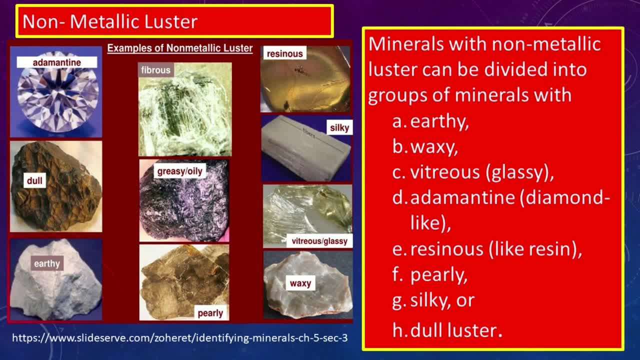 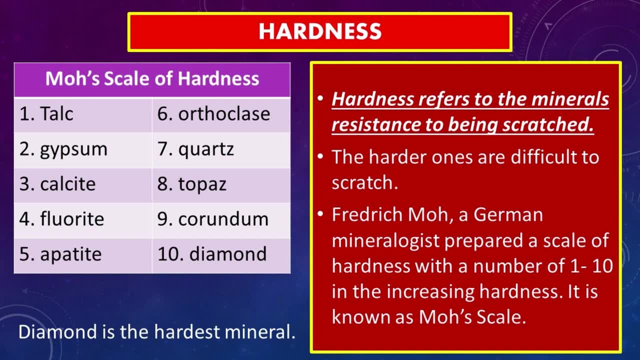 e Resinous or like resin, f Pearly, d Silky or e Dull lustre. The next physical properties of minerals is the hardness. Hardness refers to the mineral's resistance to being scratched. The harder ones are difficult to scratch. 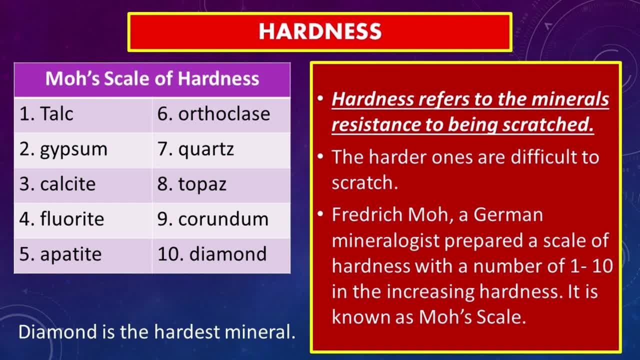 Frederick Moe, a German mineralogist, prepared a scale of hardness with a number of 1 to 10 in the increasing hardness. It is known as Moe's scale. The table shows Moe's scale indicating minerals and their hardness. 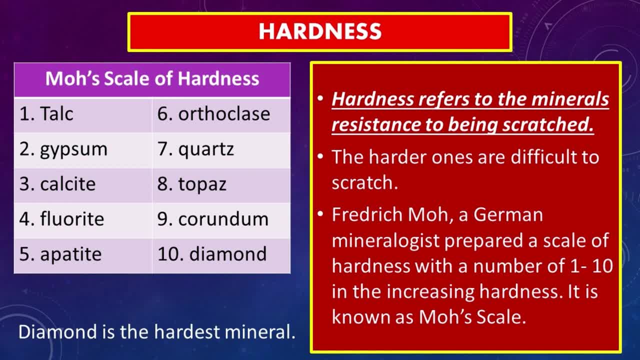 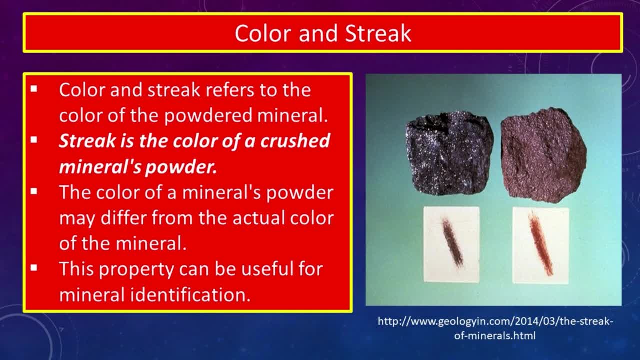 So the hardest mineral, according to Moe's scale, is diamond. Next we have the color and streak. Color and streak refers to the color of the powdered mineral. Streak is the color of a crushed mineral's powder. The color of a mineral's powder may differ from the actual color of the mineral. 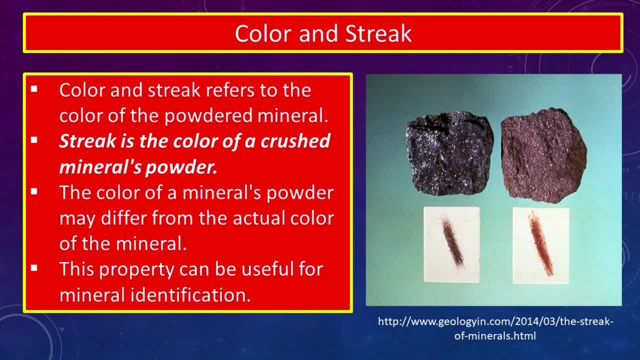 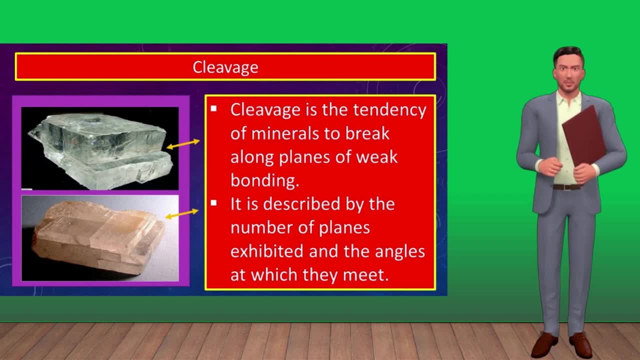 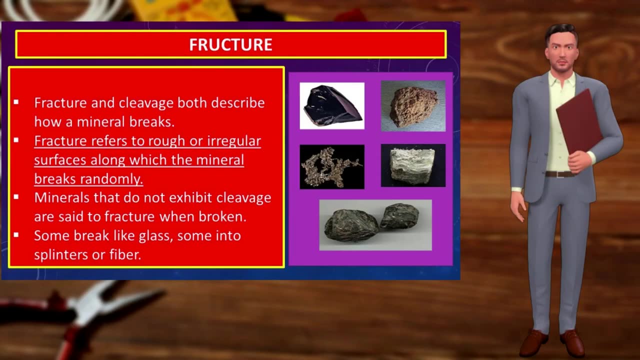 This property can be useful for mineral identification. The cleavage: Cleavage is the tendency of minerals to break along planes of weak bonding. It is described by the number of planes exhibited and the angles at which they meet The fracture. Fracture and cleavage both describe how a mineral breaks. 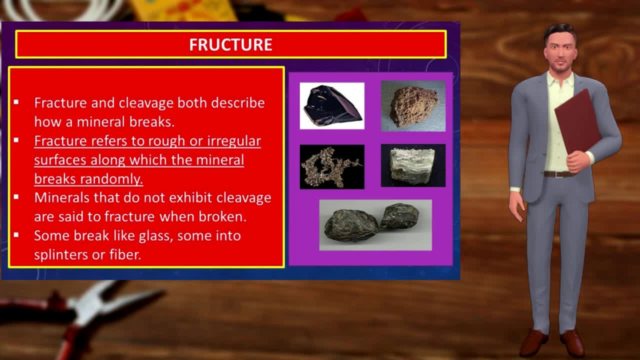 Fracture refers to rough or irregular surfaces along which the mineral breaks randomly. Cleavage refers to flat planes along which some minerals break. Minerals that do not exhibit cleavage are said to fracture When broken. Some break like glass, some into splinters or fiber. 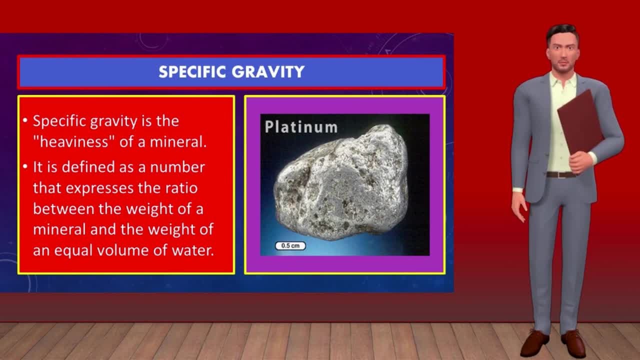 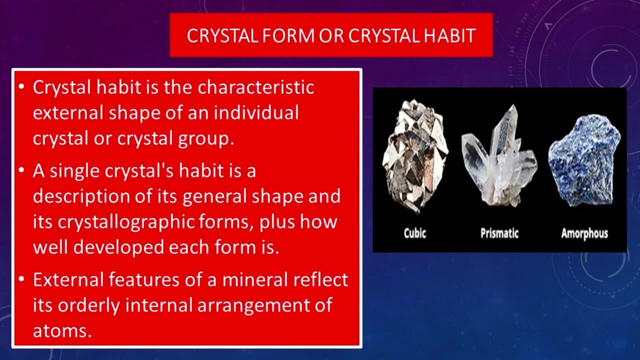 Next, the specific gravity. Specific gravity is the of a mineral. It is defined as a number that expresses the ratio between the weight of a mineral and the weight of an equal volume of water. The last physical properties of minerals is the crystal form or crystal habit. 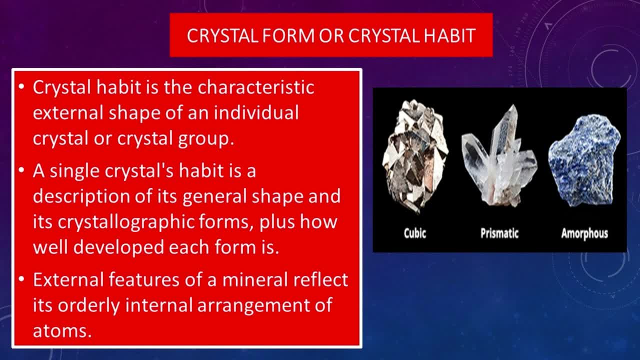 In mineralogy, crystal habit is the characteristic external shape of an individual mineral. A single crystal's habit is a description of its general shape and its crystallographic forms, plus how well developed each form is. External features of a mineral reflect its orderly internal arrangement of atoms. 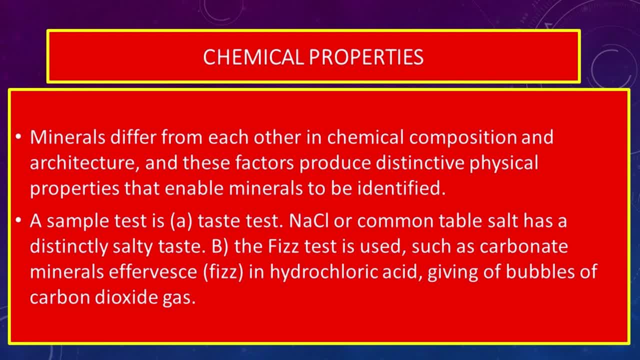 And finally we have the chemical properties. Minerals differ from each other in chemical composition and architecture, And these factors produce distinctive physical properties that enable minerals to be identified. A sample test is a taste test. Sodium chloride or common table salt has a distinctly salty taste.